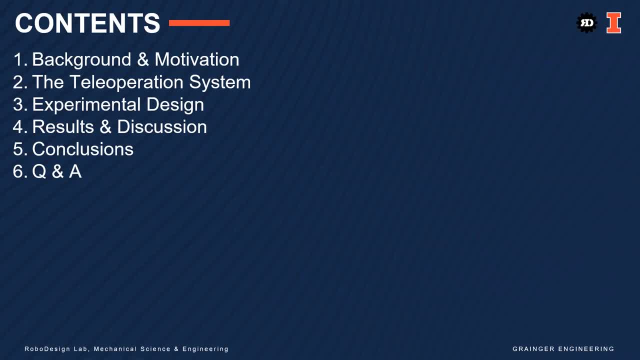 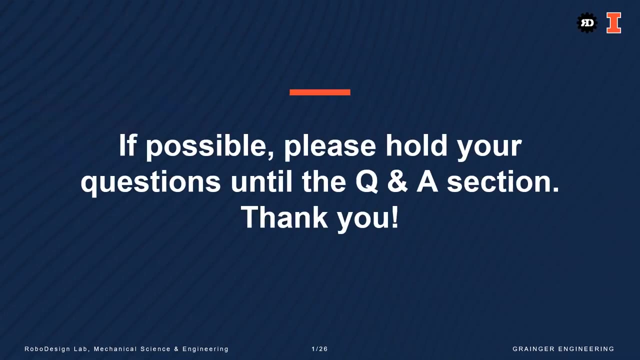 First I will begin with the background and motivation. Then I will introduce the system we studied and the experiment with which we studied the system. Lastly, I will present and discuss about the experimental results and answer your questions. As a disclaimer before we start, please hold your questions until the Q&A section, if possible, due to the time constraint of this presentation. 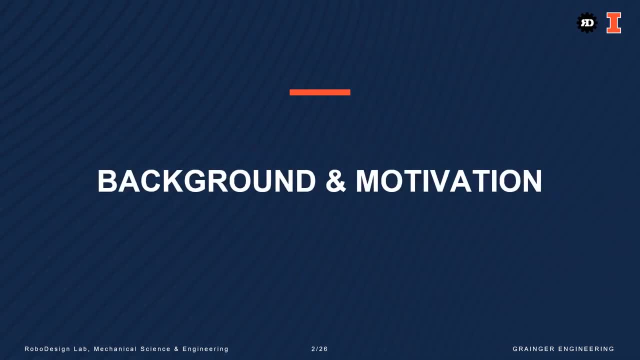 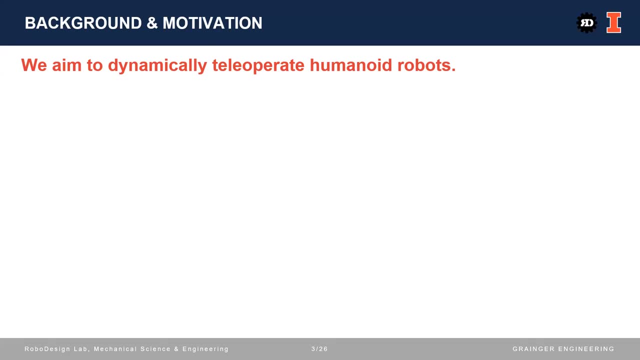 I appreciate your understanding and cooperation. Now let's get started. Let's begin with the background and motivation. Our lab's aim is to dynamically teleoperate humanoid robots. Why teleoperation? Because teleoperation can harness human planning intelligence to enable machines to achieve sophisticated tasks that current autonomous machines cannot. 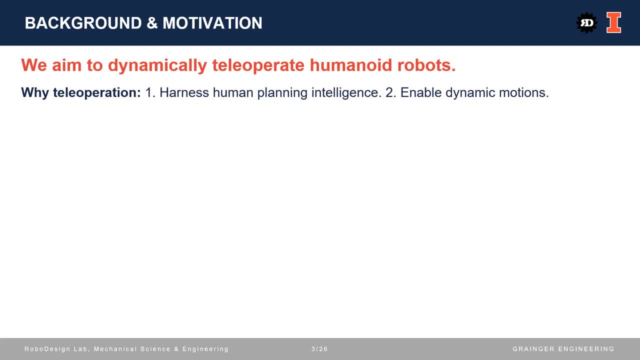 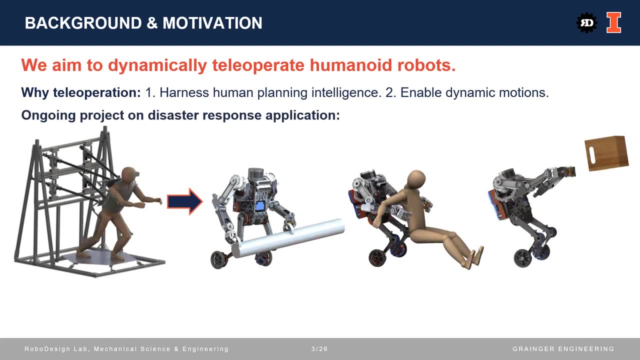 As a benefit of the human planning intelligence, harnessed teleoperation has the potential to enable very dynamic motions of humanoid robots. More specifically, our lab has an ongoing project on disaster response or application. In this project, we aim to use a human pilot and a human-machine interface to teleoperate a humanoid robot to perform very dynamic tasks, such as using a heavy object to slam a door, rescuing a human and throwing a heavy object. 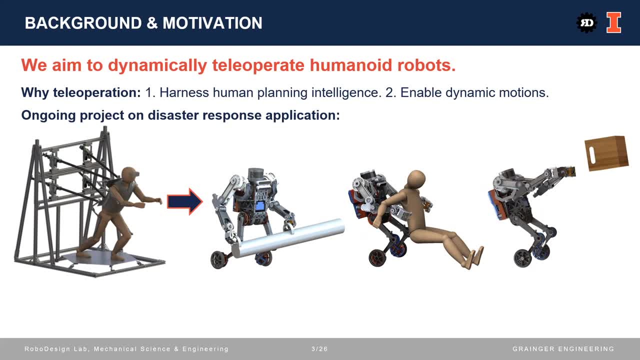